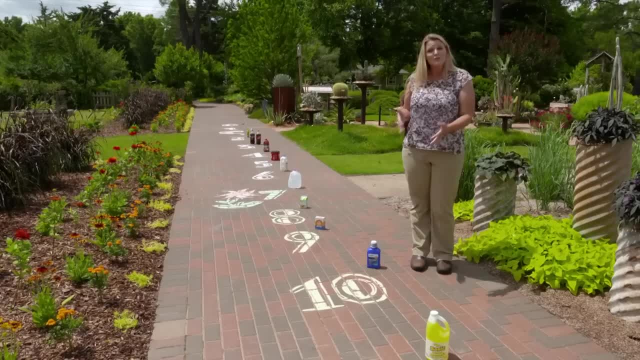 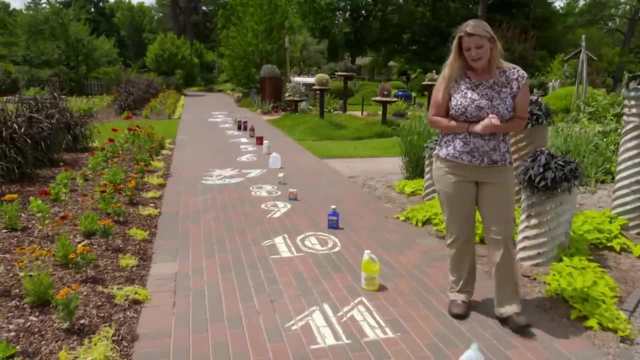 We have milk of magnesia, which is an antacid, So we often take this to help balance the stomach acids. At 11, we have ammonia that's used for cleaning, As well as 12,, we have soapy water. 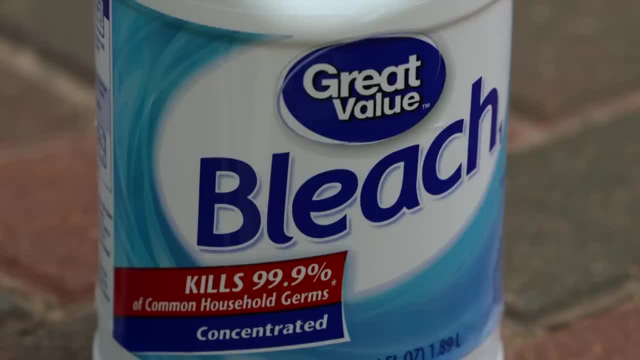 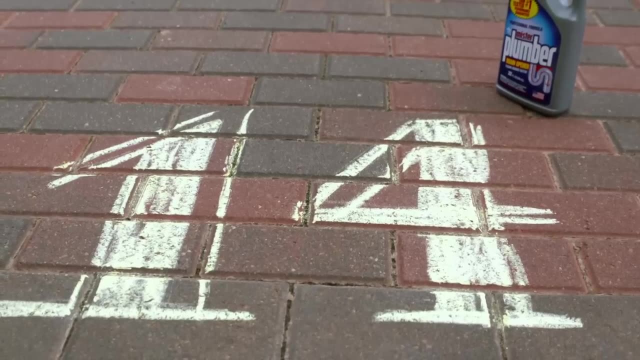 13,. we have a lot of our bleaches, And then, finally, some of our most corrosive bases is our drain cleaners at 14.. So what does all of this have to do with gardening? Well, just like our own bodies can get upset when our pH is off, so can our plants in our 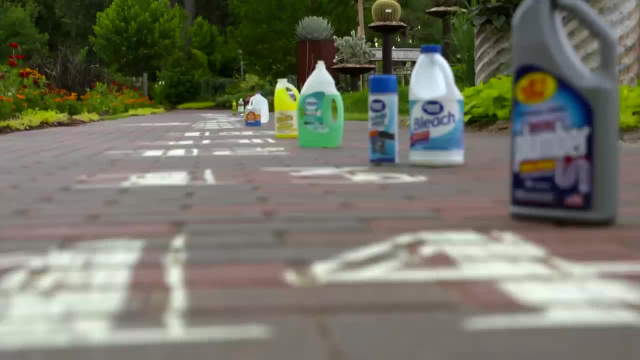 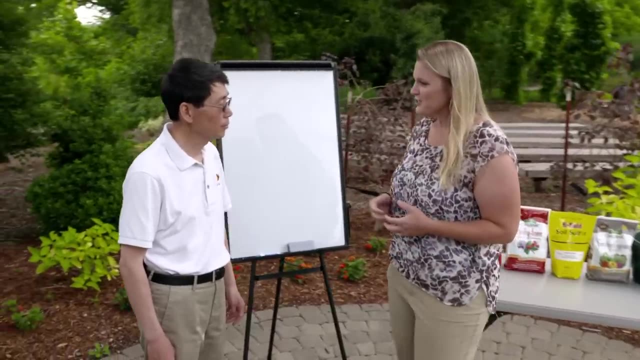 garden. So for more information, we're going to go talk to the expert, Dr Zheng. thank you for joining us. again, We're going to talk about pH. Can you explain a little bit of the science behind pH? Well, I'd be happy to. 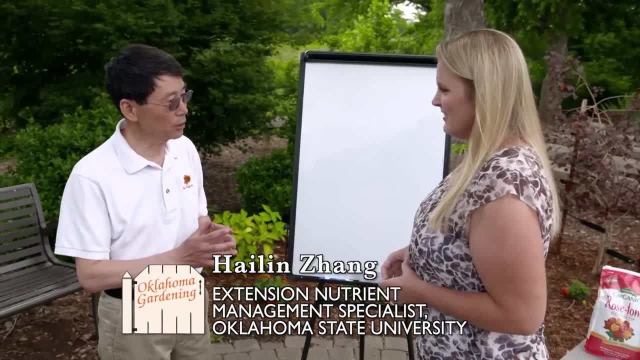 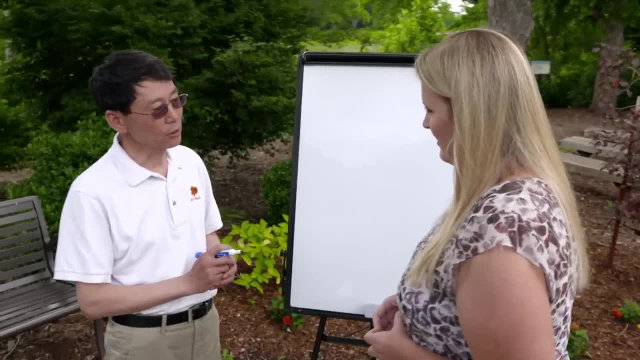 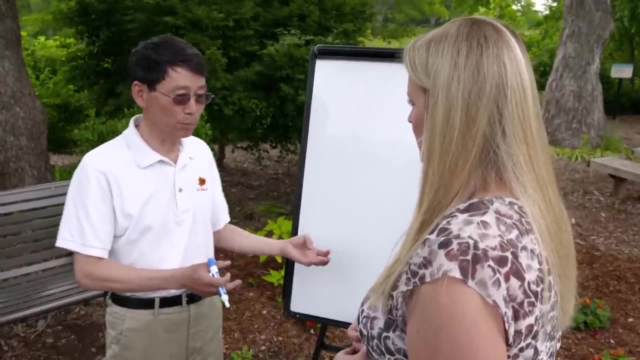 pH is one of the most important tests in the routine package we talked about the last time. So pH basically is It's measuring the soil acidity or alkalinity in the soil. It's very important. It's just like our blood pressure: It can't be too high or too low. 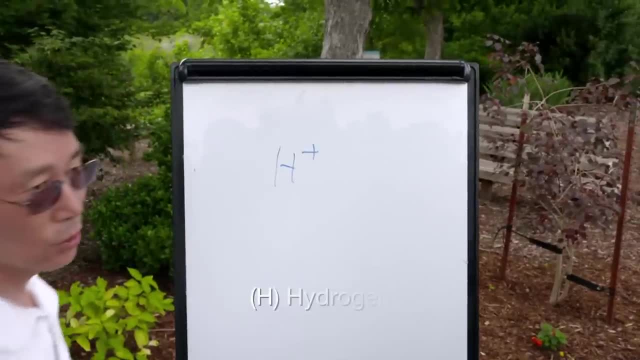 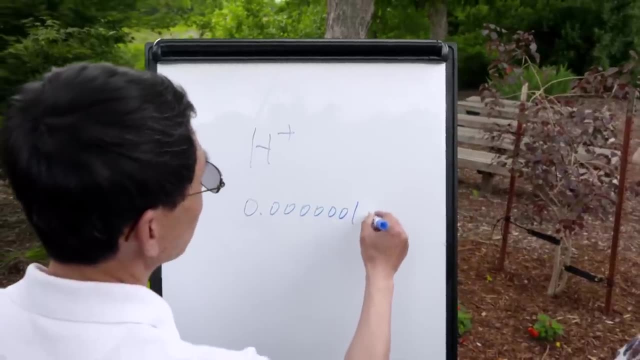 Basically, the acidity is the hydrogen ion in the soil. okay, It's very low. Typically it's like 0, 0, 0, 0, 1 molar, right, Okay. Or 10 to the minus 7.. 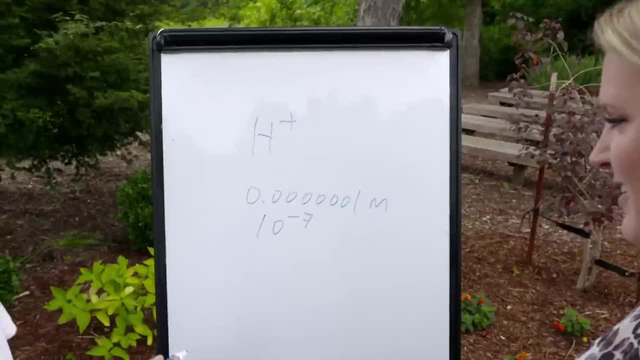 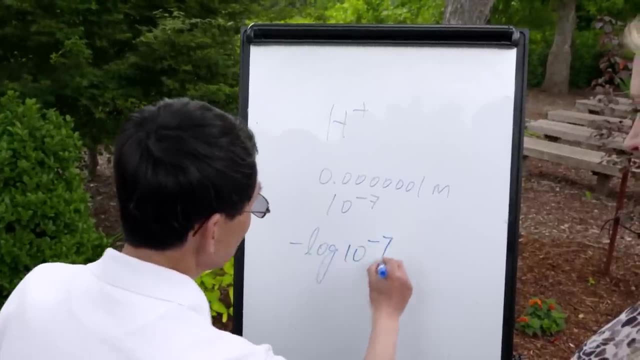 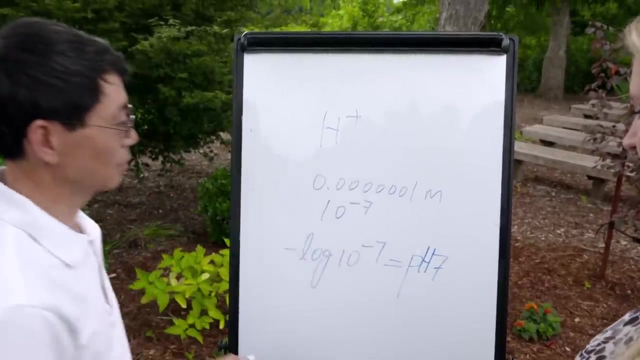 That's how low it is. Well, it's very tedious to write all this amount. Yeah, Yeah, That's right. So people used a simple negative log to express that That word equals 7.. So they put a pH there: pH 7.. 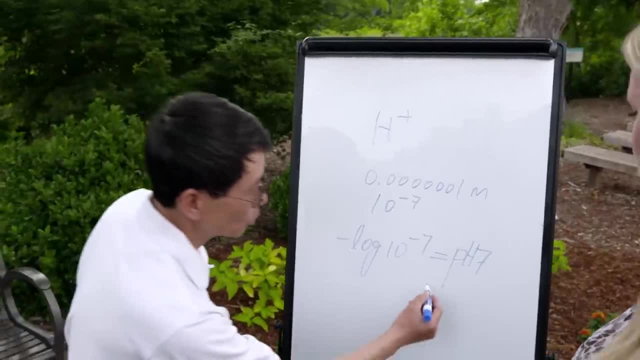 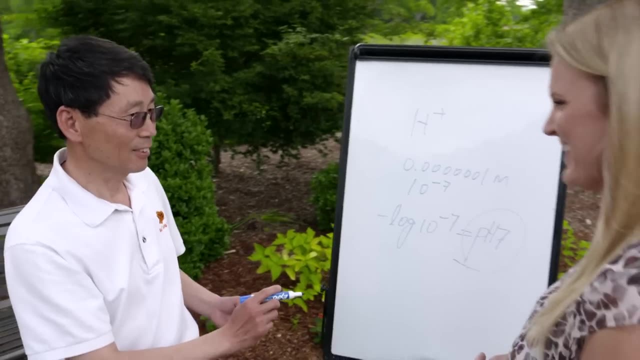 This is how pH is expressed In the laboratory. we do all this conversion. We tell you your soil pH is Okay. So you give us whole numbers to work with. Yes, Typically it ranges from 0 to 14.. However, Most plants like the neutral range 6.5 to 7.. If the pH is too low, you have a very serious problem. When it's too high, some of the nutrients are not available to plants. They're like rocks precipitating the soil. 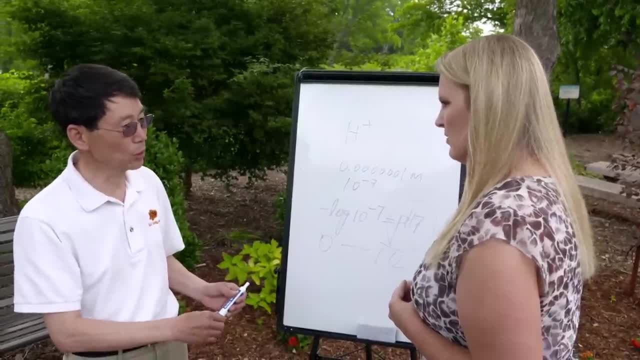 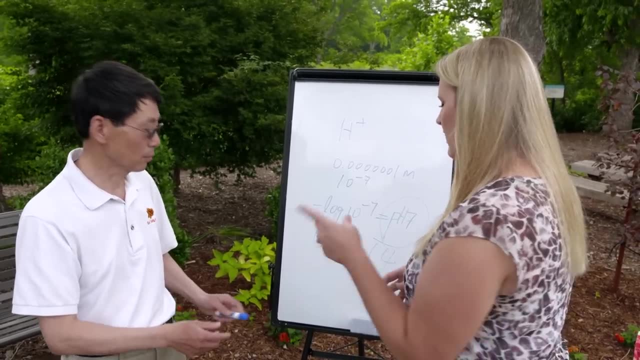 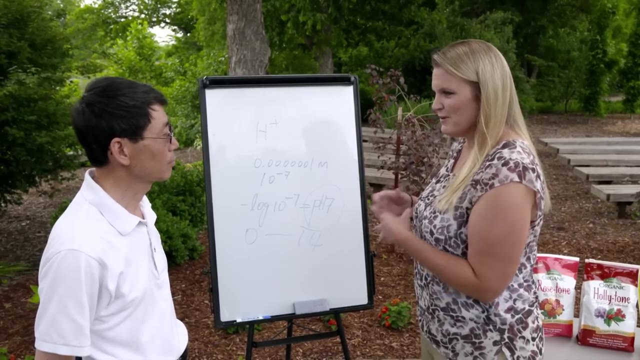 This is why we like homeowners to pay attention to pH. If there's a problem, we can correct the pH using the products available to us. Well, I think what you said about nutrients being tied up is kind of an important thing, because a lot of times we don't realize that we might be fertilizing but it might not be accessible. 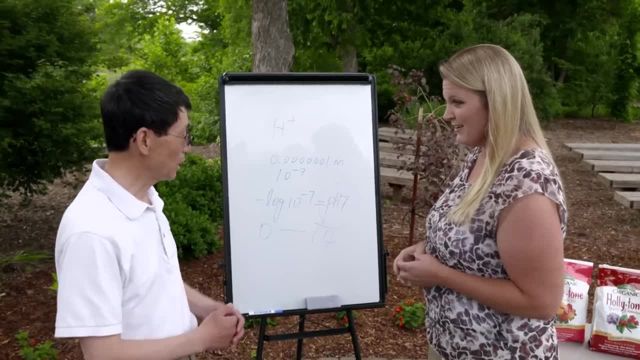 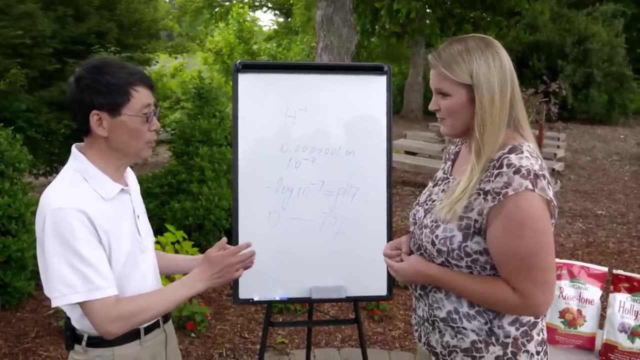 to the plant if your pH is off. You're exactly right. You know some of the nutrients like iron, zinc. those are micronutrients. When the pH is about 8 or 7.5, they become solids. So that's why we see iron chlorosis and other problems. 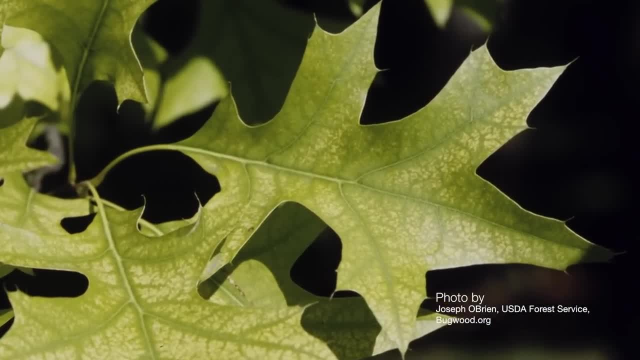 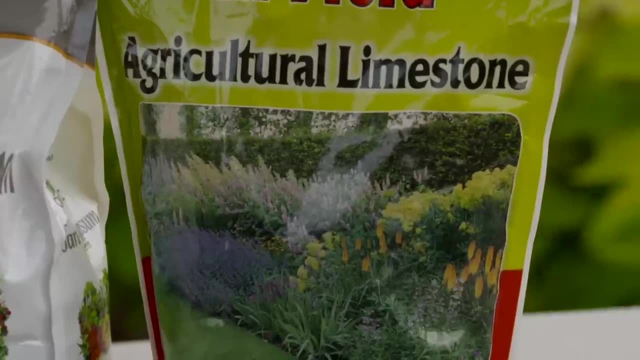 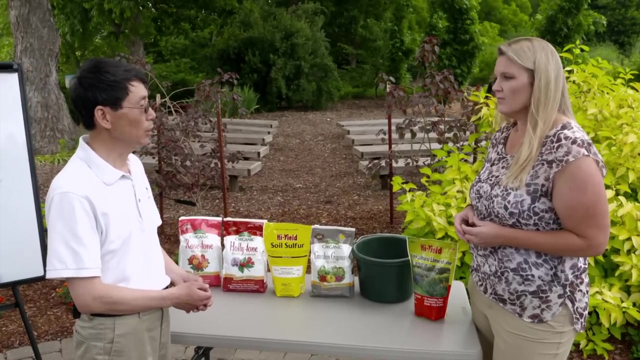 A lot of our pin oaks have that problem Exactly. So if we find out we have a low pH, what do we need to do? We need to add some lime. Well, lime is a caustic material. It brings the pH up or neutralizes soil acidity. 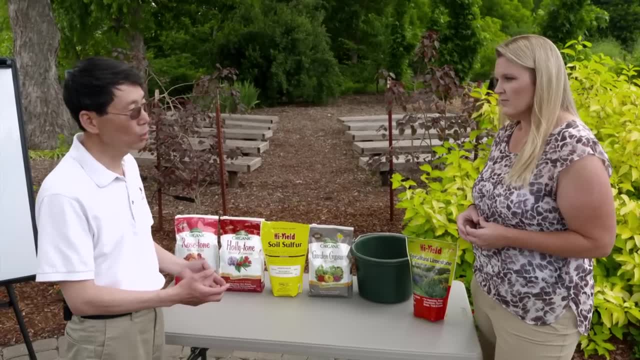 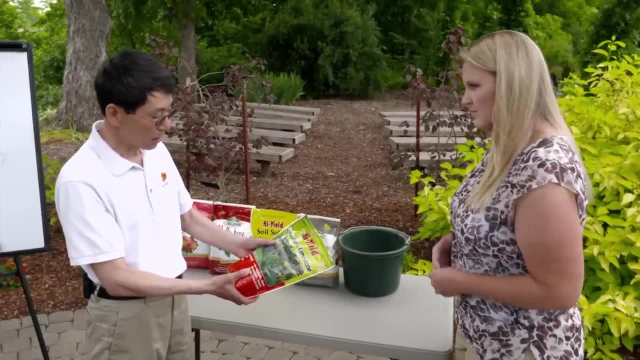 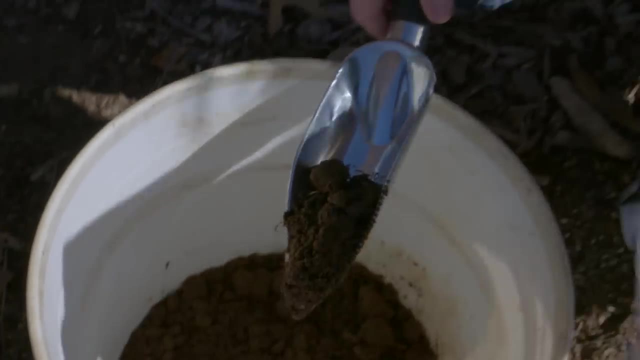 So if a soil has a pH like 5, which is low to most plants, then we add agricultural lime to neutralize it. Well, how much to apply? First of all, It depends on soil pH. That's why people need to do a soil test. 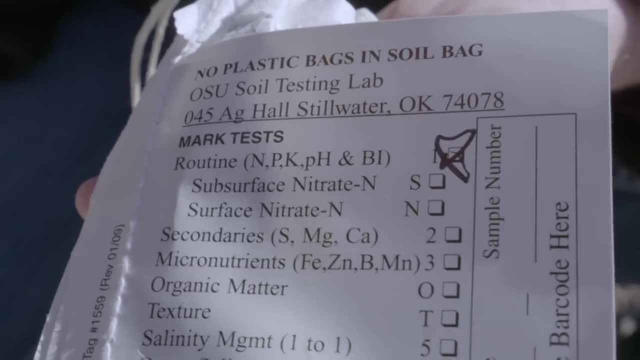 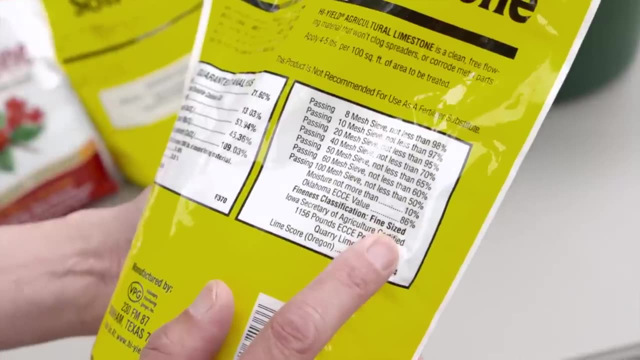 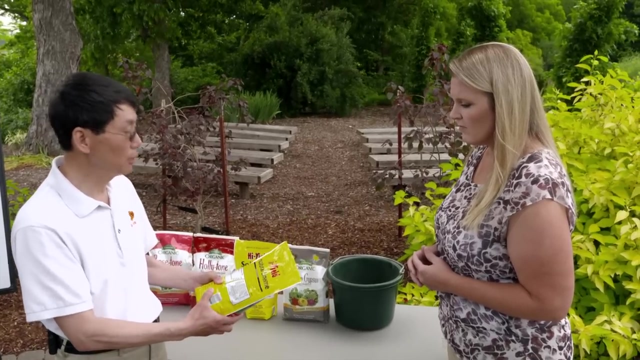 And that's on your basic soil test. Yes, Your routine soil test. Then you find the product. The product will tell you the purity of this. This is like 86%. If you need 10 pounds, you need a little bit more than 10 pounds to supply the needed active. 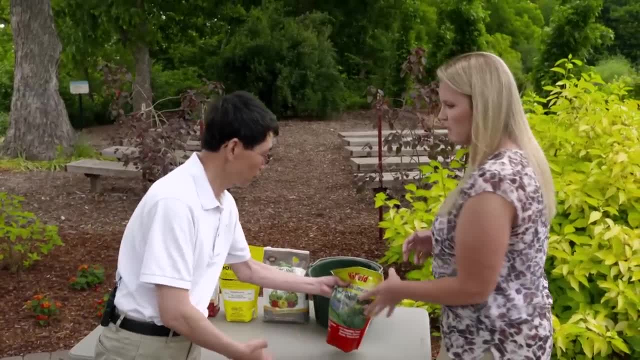 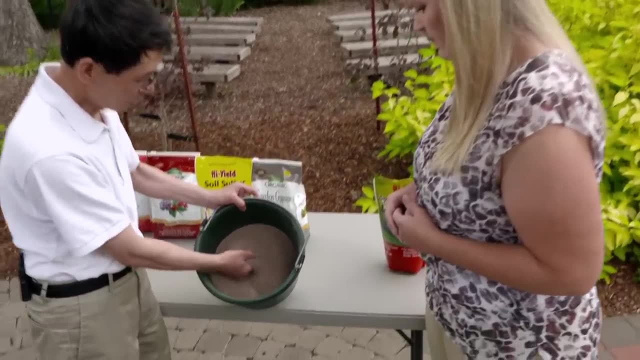 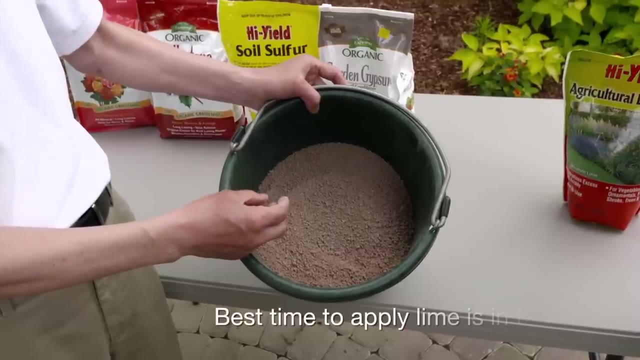 ingredients. Okay, So you would calculate this the same way you would calculate your nitrogen needs. Yes, So people can go to the garden center find that this is palletized lime. Now, what is a good time to apply? Typically, it's in the fall. 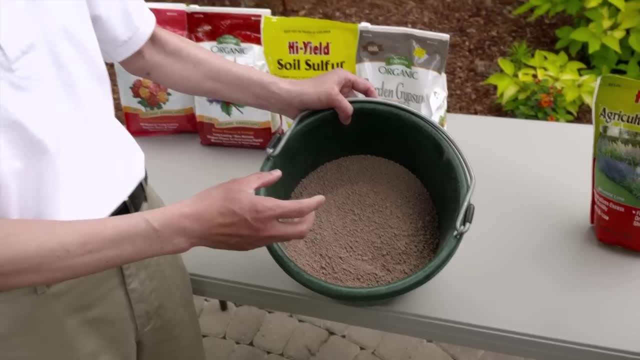 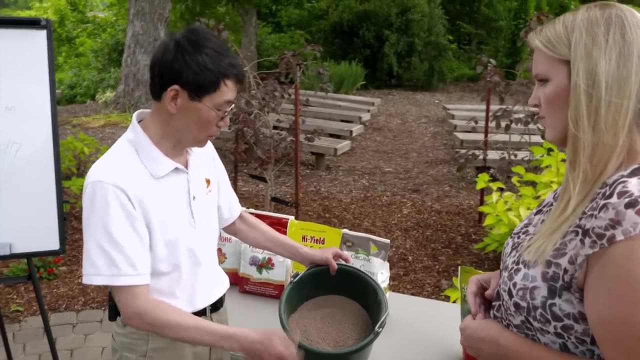 It takes time for the lime to react with the soil to raise the pH. So by the time you do a spring planting, the soil pH should be neutralized to the right range. So if people follow our recommendation it's very easy to get the pH corrected. 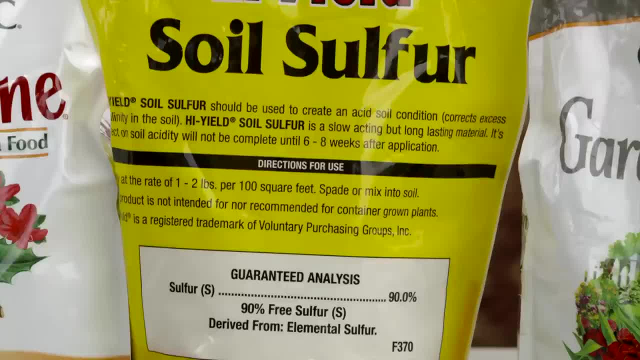 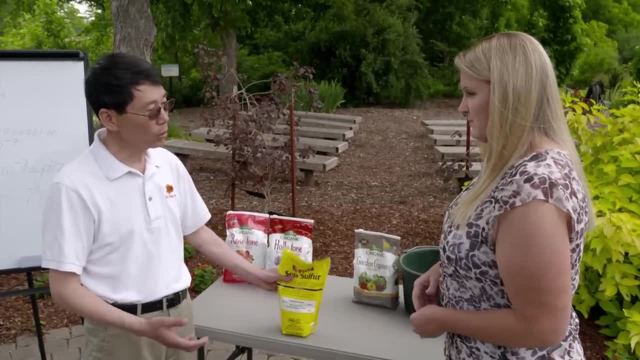 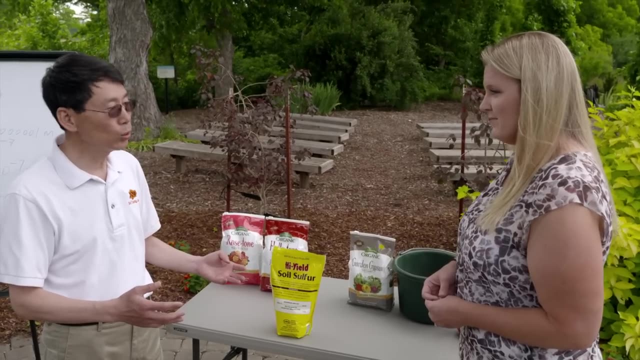 Okay, And then we've got some sulfur here, which is what you would put down if your pH was too high. Exactly, Most plants can tolerate a wide range of pH, but some plants, like azalea or blueberry, they can grow at normal pH, like six or seven, but they just don't bear fruits very well. 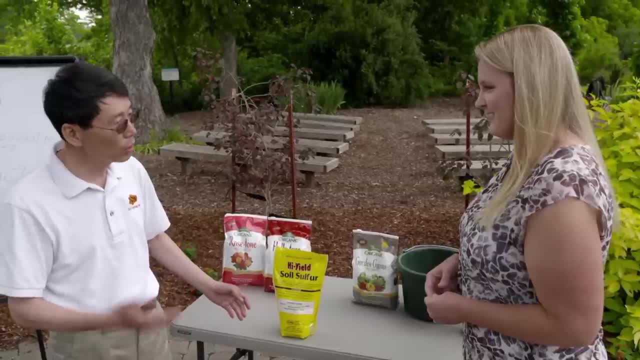 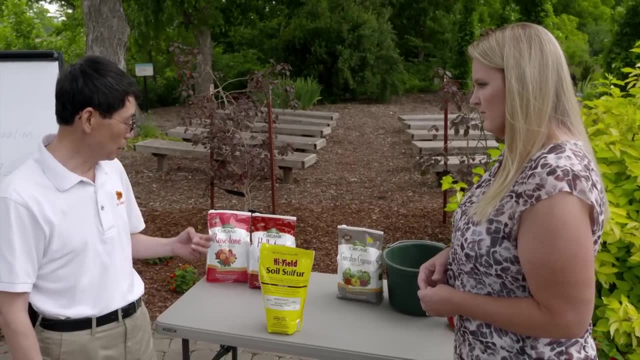 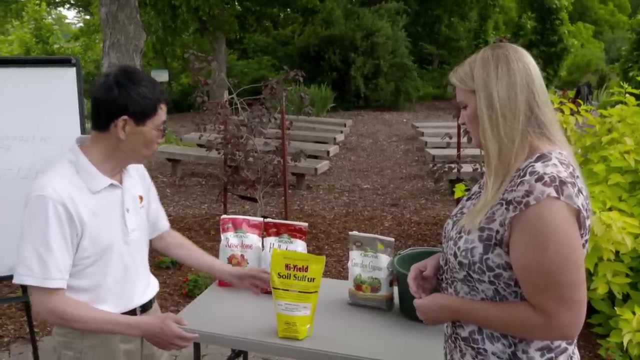 So in that case for a serious gardener, they would like to lower the pH or add acidity to the soil. There are several products available, like alum- It's aluminum sulfate people can use to acidify the soil, but most common is this sulfur. 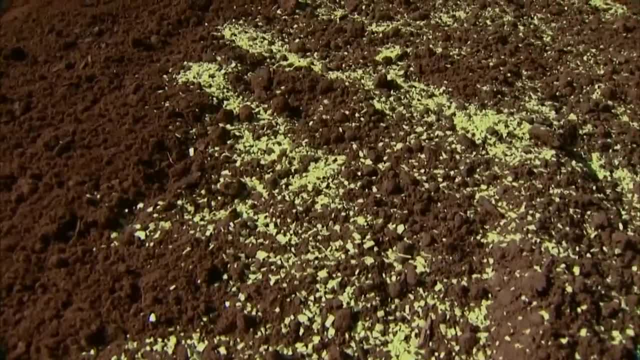 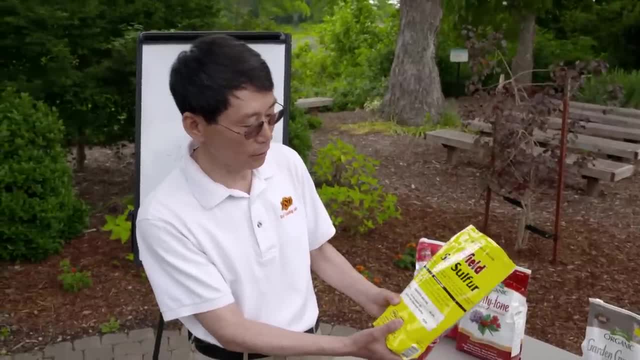 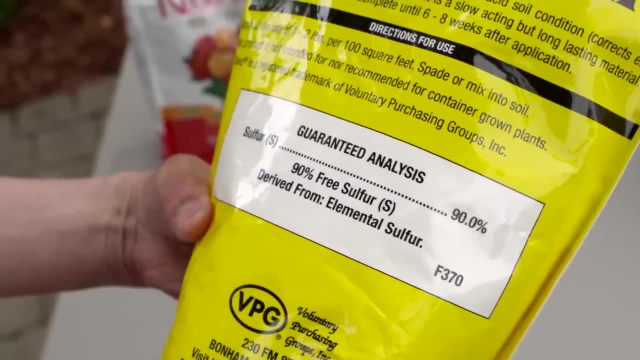 After we put in the soil, the microorganism will oxidize to sulfuric acid. This is how to add acid to the soil to neutralize the alkalinity Like this. one has 90% of sulfur in this product. It's very effective. 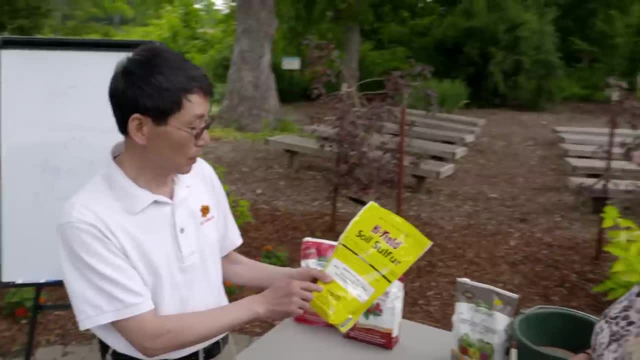 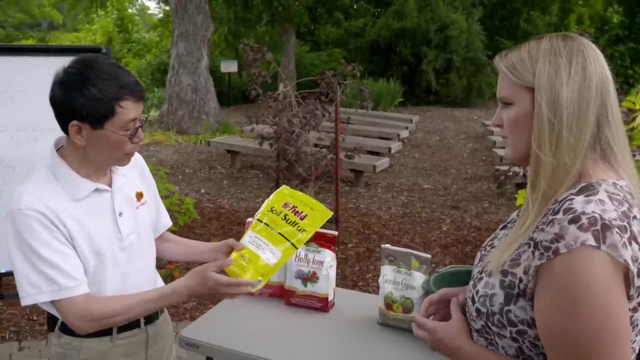 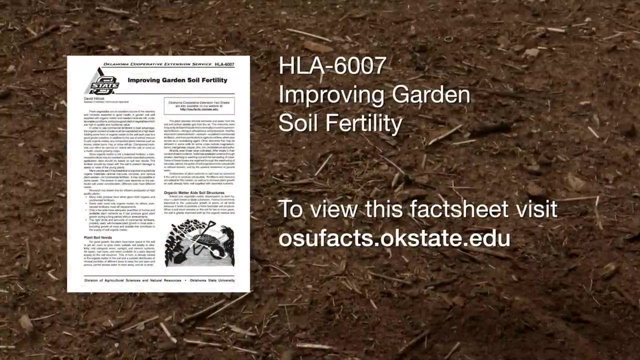 You want to make sure to water these in correct? Yes, This can add it ahead of time. It reacts with the soil very slowly, so you need to be very patient. There's a fact sheet. I think the title is: improve garden soils has an instruction how much to apply. 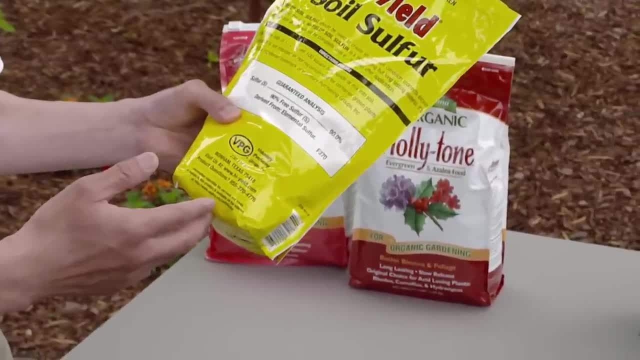 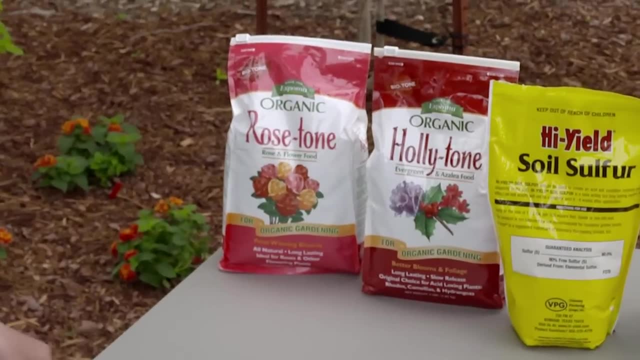 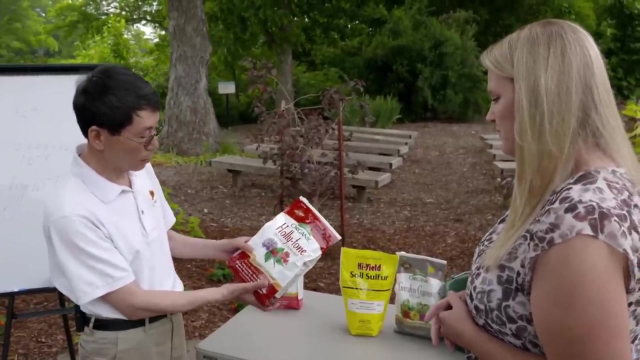 Typically just two to three pounds per 100 square foot. Okay, But people need to analyze the soil, probably frequently, to check to see the pH level. Some of the fertilizers, like this one, is labeled for azalea- also good for blueberry. 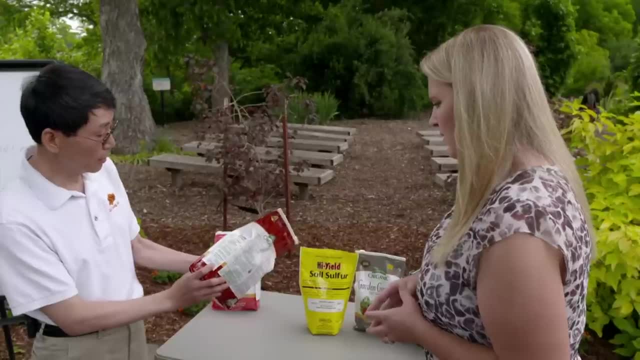 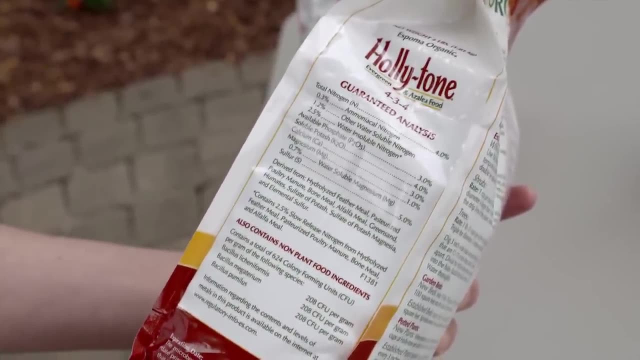 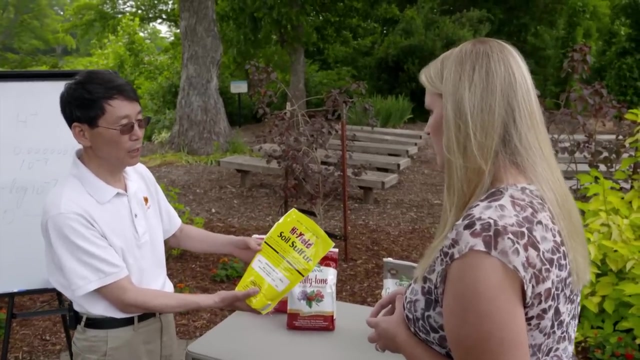 The reason for that is it contains not only the nutrients like nitrogen, phosphorus, potassium, It also contains 5% of sulfur. Okay, This sulfur would act to neutralize alkalinity. like this, It's a pure sulfate compound. This might be something if you just need to slightly adjust your pH lower, whereas if 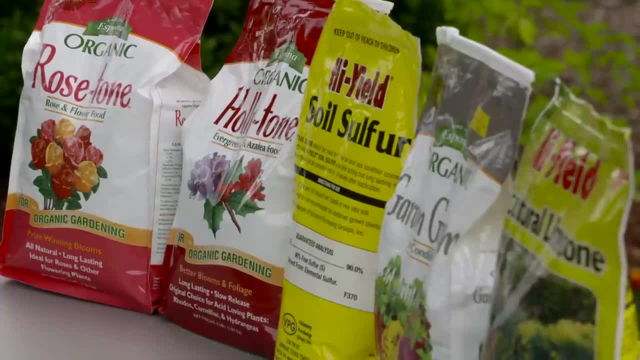 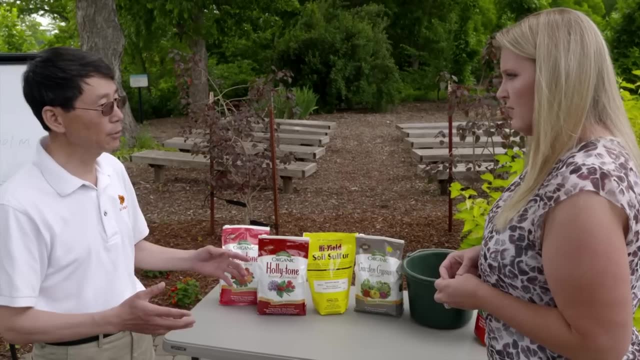 your pH is more alkaline and you need to go more drastically, then you can use sulfur Right. These plants like pH about 5. If you have a pH at 8 right now, it will take quite a bit of sulfur to do that.